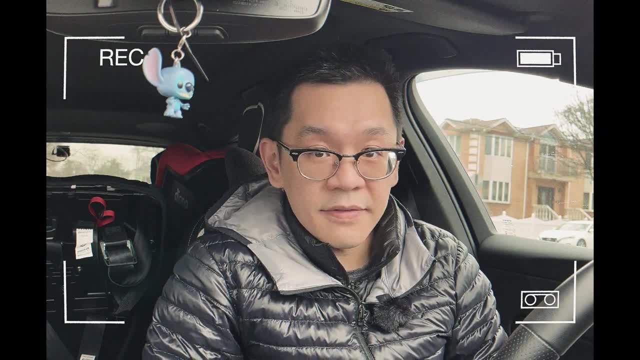 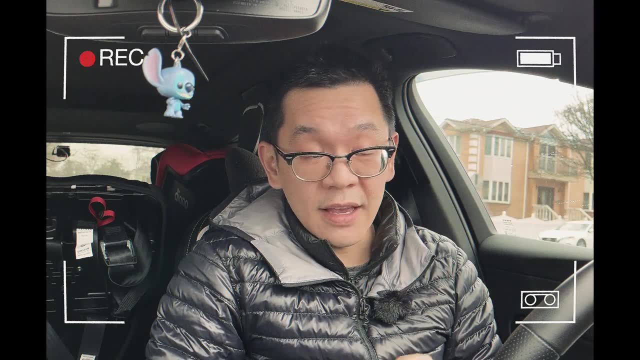 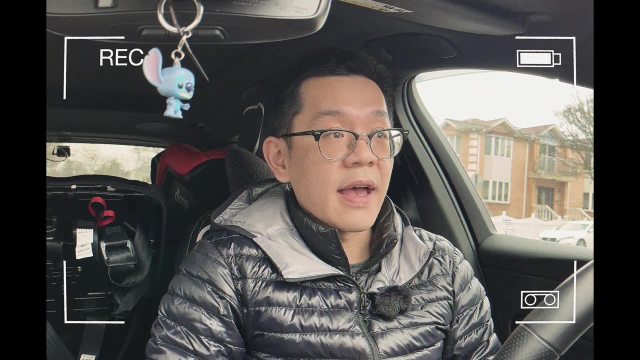 What is going on, guys? So in today's video I want to go ahead and hit up a strip of dealerships and make sure that we're making the right choice and going for a minivan. So what we're going to do today is look at or check out all three row SUVs as much as we can to make sure that we're. 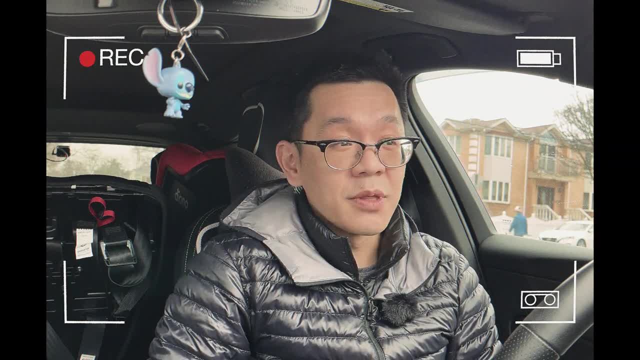 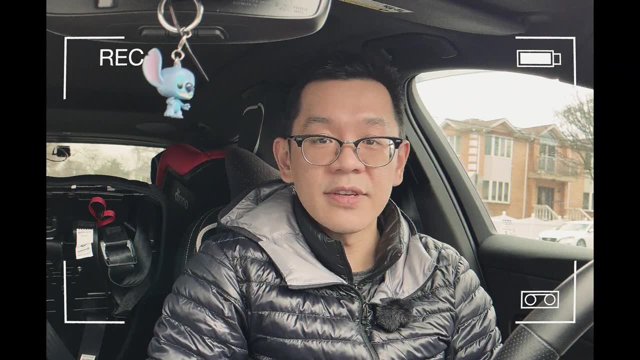 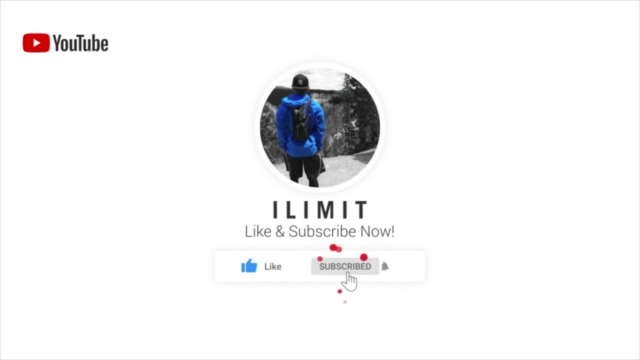 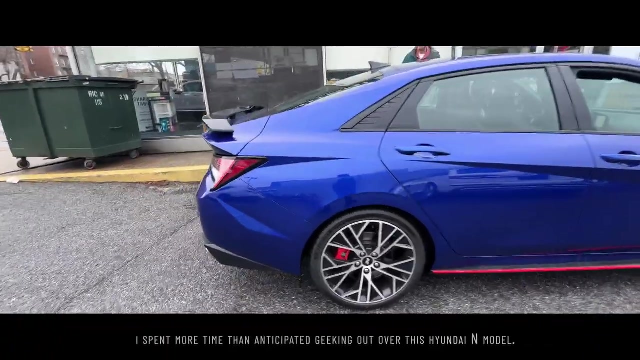 not missing out on anything or if we're going overboard with the minivan allocation and decision. So stick with me. I hope you guys join me around this adventure today and let's go. I'm going to have to stop this video by taking a look at this. Elantra N. This sounds nice. 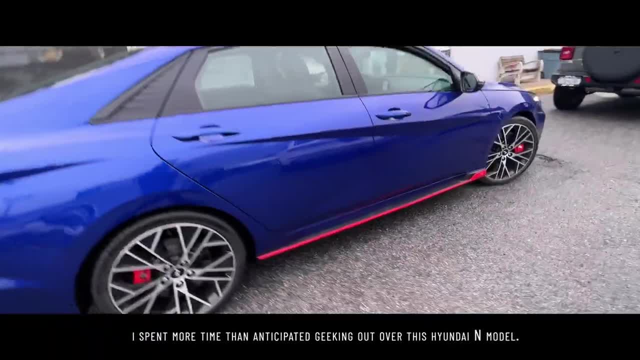 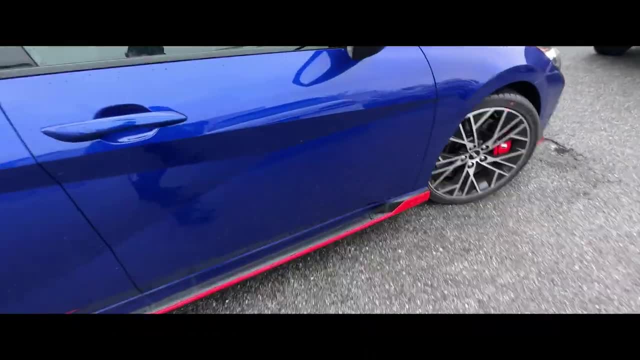 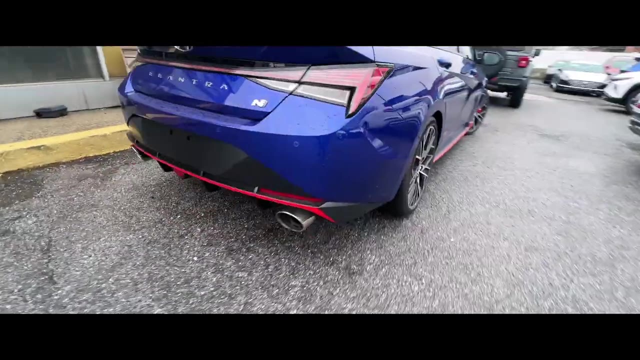 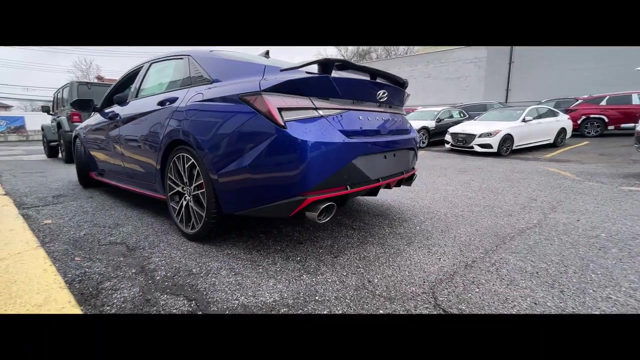 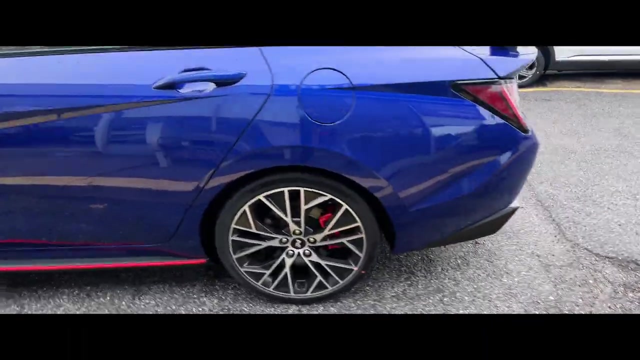 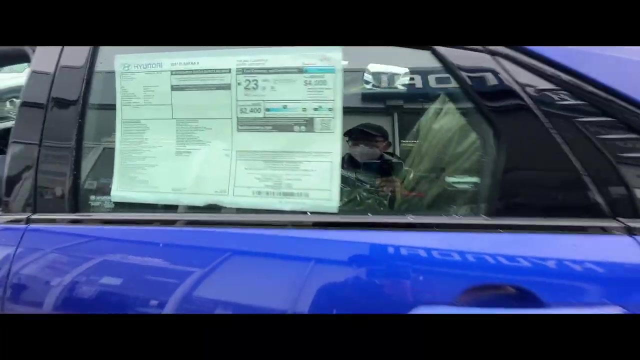 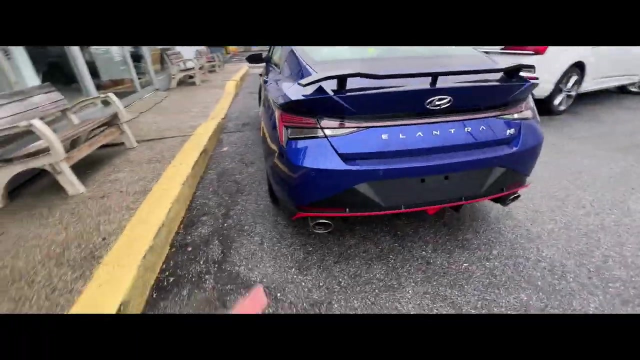 Wow, this is a nice car. Nice, I like it. Is that the DCT? Yeah, Now guys, this is a stock system. Sounds nice, Perfect, MSI, MSI, MSI SRP 35 440.. This is a 2023 model. This is in blue. Wow, look at these exhaust tips. 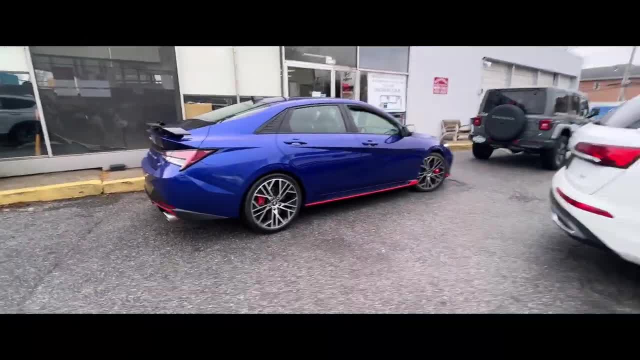 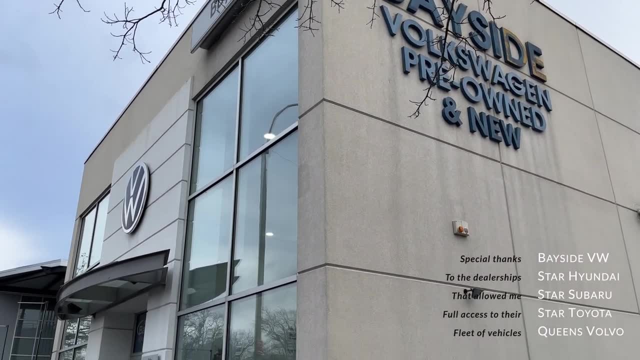 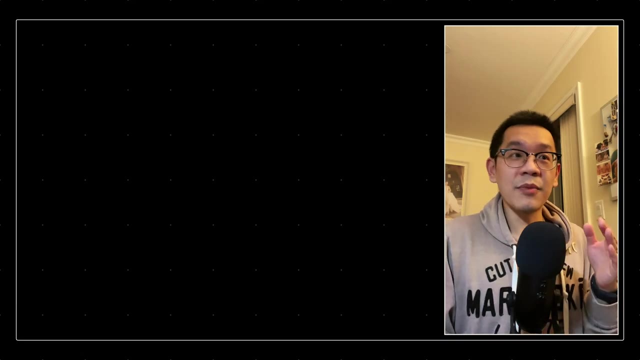 This is nice. All right back to an original program. All right, guys. so a change of environment. I decided to go home and do a complete analytical breakdown of why we should maybe consider a three row SUV versus a Sienna. Let's go ahead and talk about my previous video. I wanted to 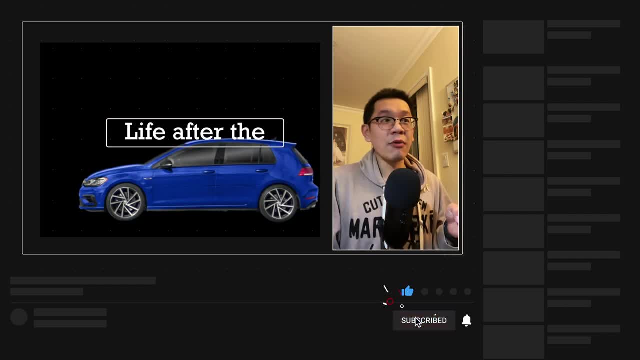 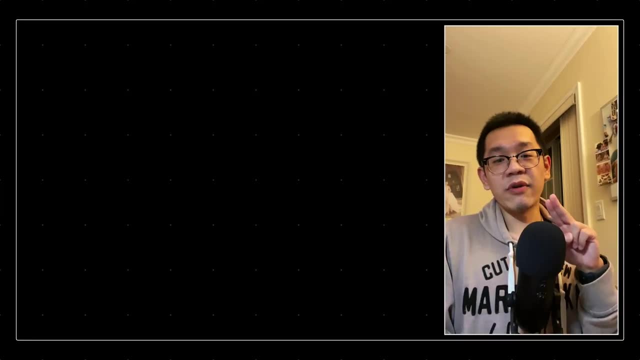 talk about the requirements, one being all-wheel drive and one being a gas efficient motor, and the Sienna versus all the other minivan options out there met two of our needs. So I decided to go ahead and do the Sienna versus the Odyssey because of the all-wheel drive again. But let's go ahead. 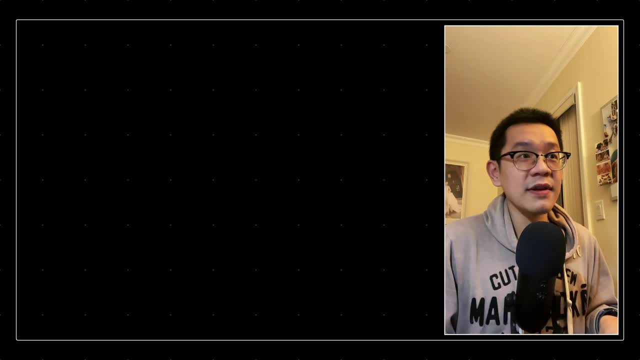 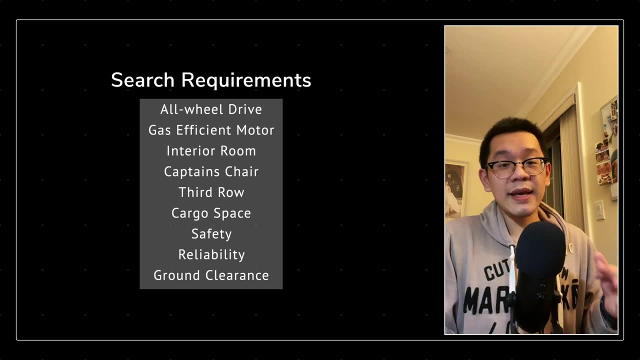 and just refresh on the requirements from the previous videos and not really particular order. but we want an interior room, increased interior room from our Golf R that we started with. We want a captain's chairs for ease of going in and out and also taking care of our girls. 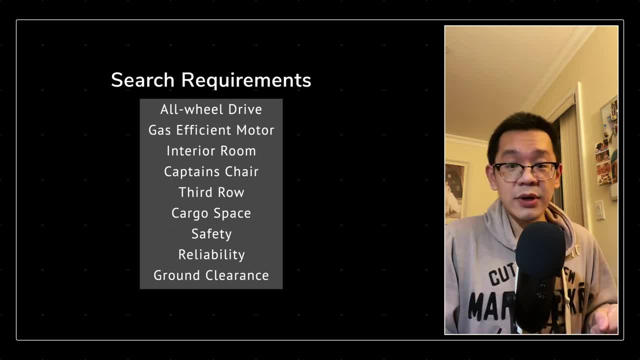 We want a third row for more passengers, for more field trips, for more road trips And we want a decent amount of cargo space with the third row up. We want a safety and reliability And we want it for the most part. we want a decent amount of ground clearance, So any type of 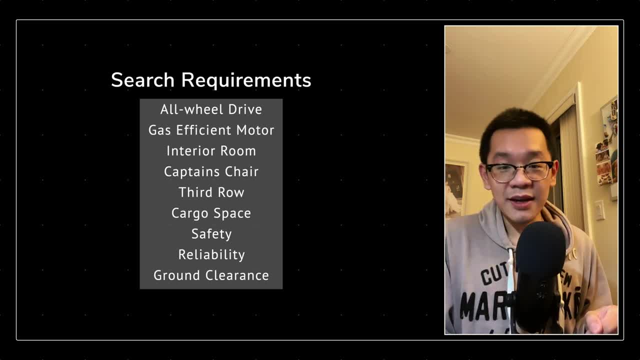 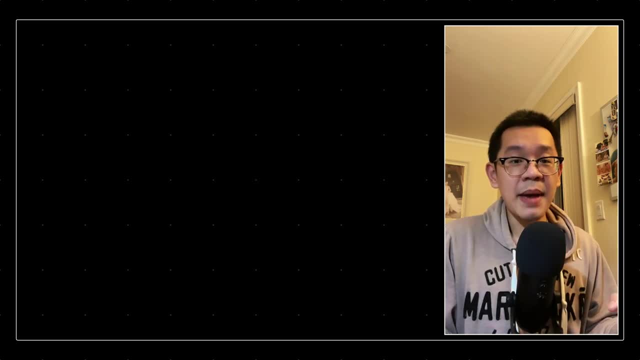 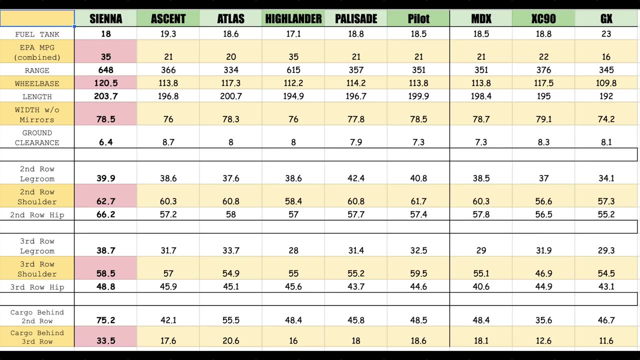 ground clearance higher than my Golf R will do the trick, but we definitely wanted something that will play nice in the snow. So, having said all that, the Sienna met all of these requirements in my opinion, But at the same time- I'm going to throw up this list right here- that we have the three-row SUV versus Sienna. 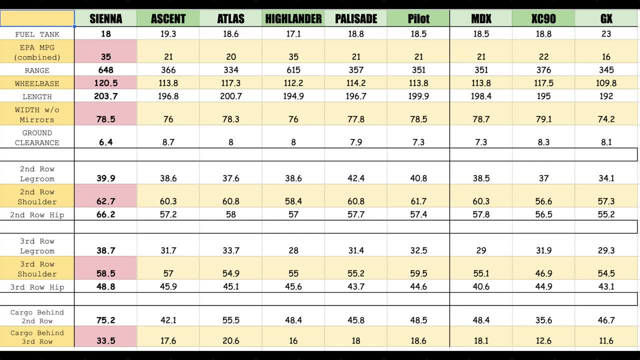 spreadsheet. Most of these contenders in front of me do meet many of these requirements and the only requirement that the only point that it doesn't meet should be the gas efficient motor. So from here I'm going to touch up on that last, because that's going to be the deciding factor. 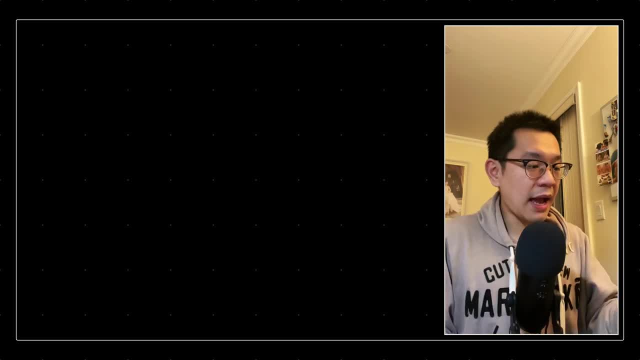 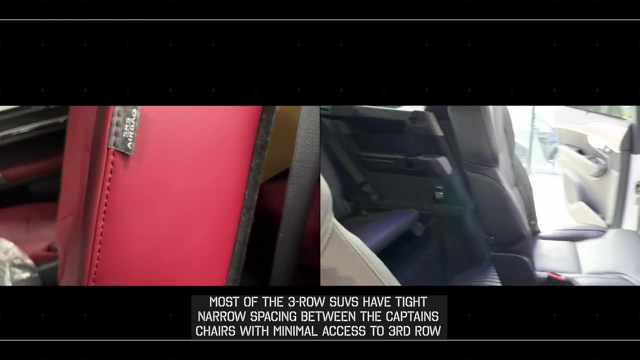 that kind of dwindles down, narrows down down our search. but as you can see from here, we're gonna go ahead and touch up on. let's see the second row shoulder room. from here you can see that well: the GX, the Highlander, the XC 90, everything else is kind of 60 inches or above all I. 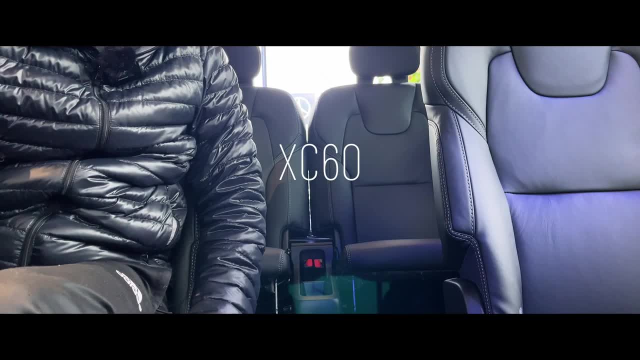 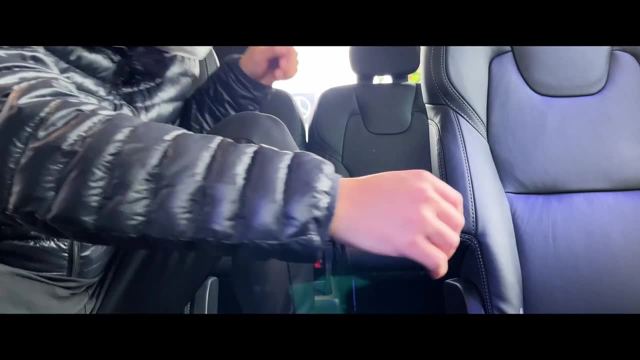 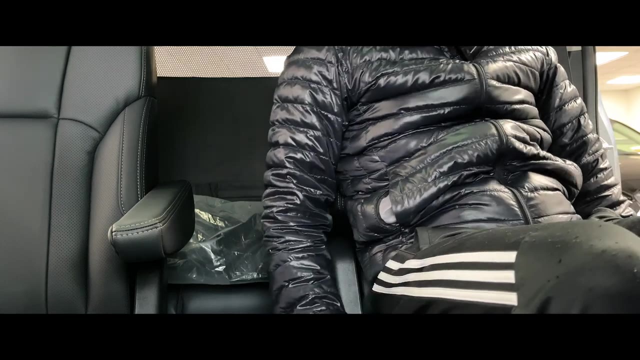 remember is the XC 90 had no armrest for the captain's chair. however, getting into the third row through the middle section, the gap it was still pretty minimal. it's a very slim and very narrow same with the ascent. even though it says sixty point three inches, from what I remember, is kind of still very narrow. 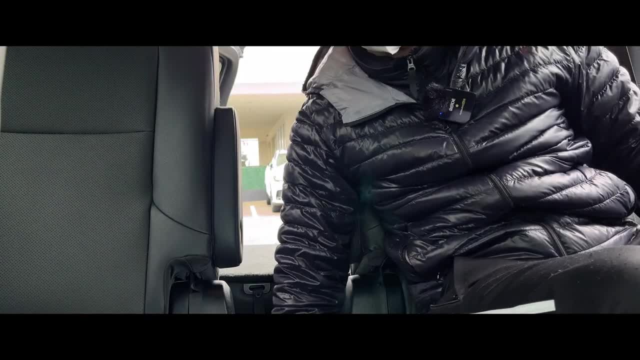 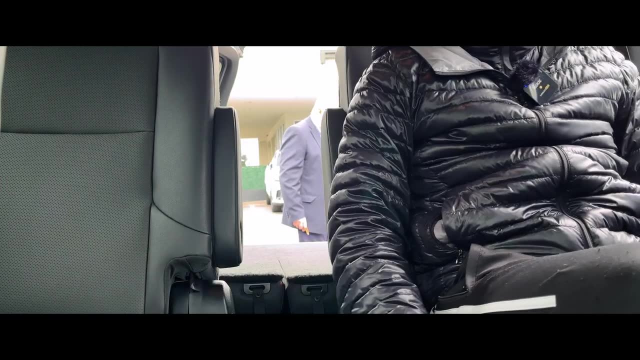 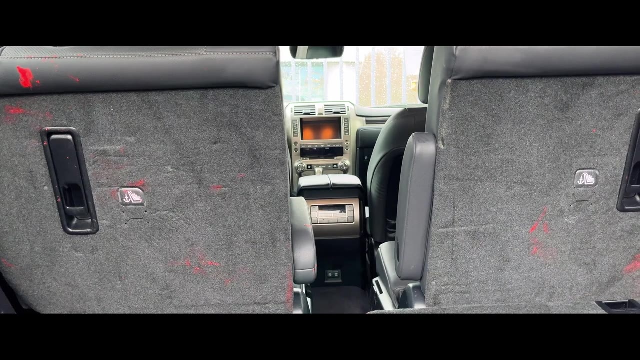 along with the, the GX, and GX was very disappointing in terms of space. it was comfortable inside but at the same time, is very it's felt very cramped. if you're going for the third row with the third row down, then yes, it felt very comfortable, like it, you know it's. it's a nice, comfortable ride. however, with the third 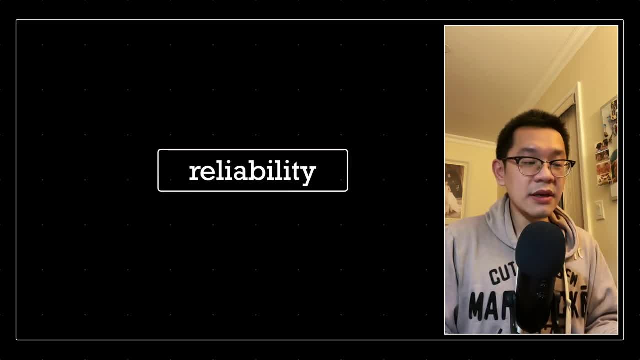 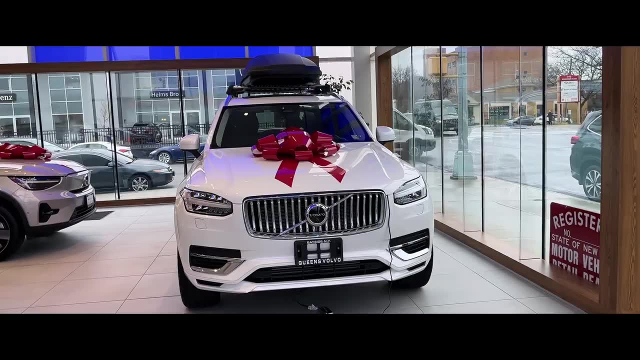 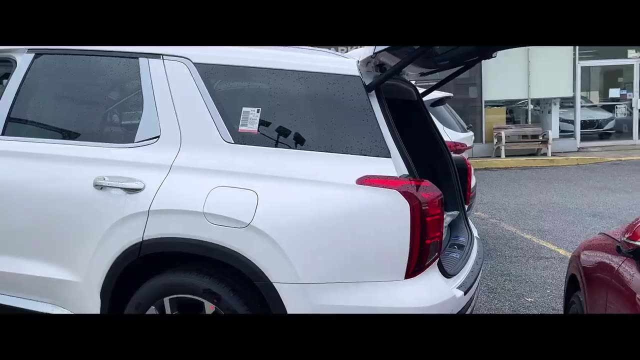 row up. it's a completely different story in terms of reliability. you have the Volkswagen, who always have the stigma of you know, not so great in terms of reliability. you also have the Volvo. be wary of the Volvo's if they're out of warranty. and you also have the Kia products from Korea, right a hundred. 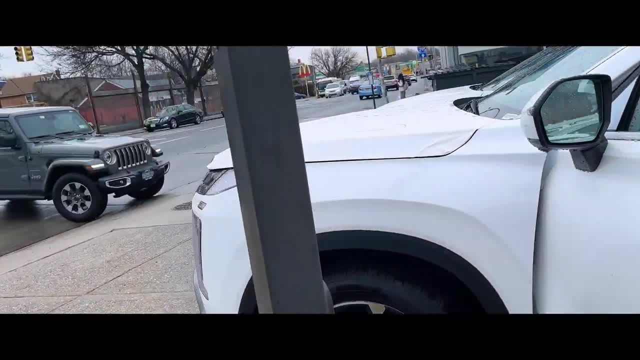 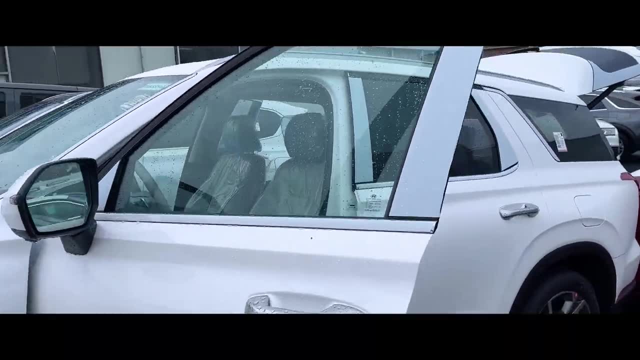 thousand mile powertrain warranty. I believe, however, a lot of people on the forums they do talk about a hundred thousand mile powertrain warranty. however, a lot of people on the forums they do talk about all these small problems that arise when it comes to problems. so I don't want to. 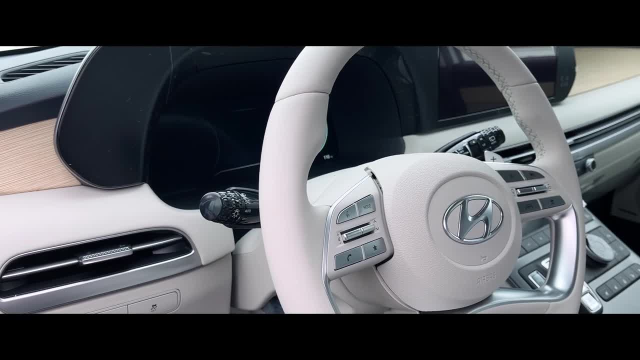 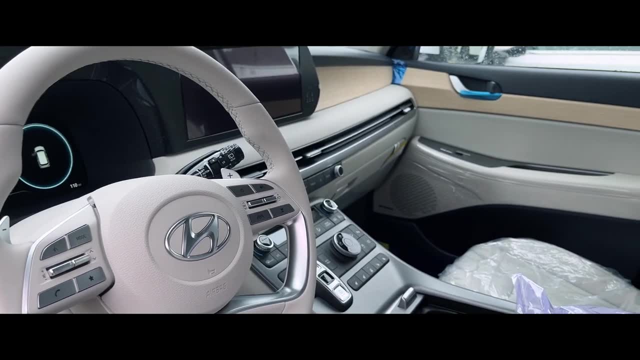 risk a chance that, but at the same time, though, let's talk about the Kia and the Telluride. they offer a ton for the money, so that's why it's here and that's why I'm very interested. now, moving on, most of these new SUVs will advertise their 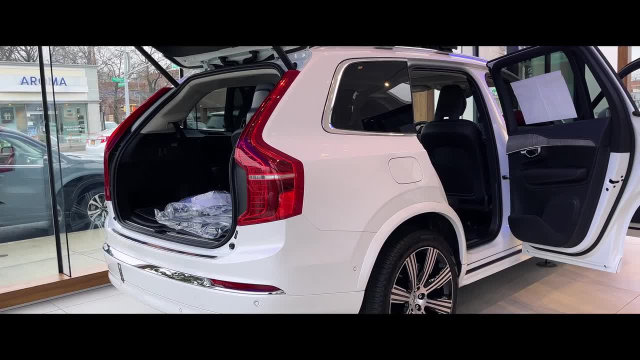 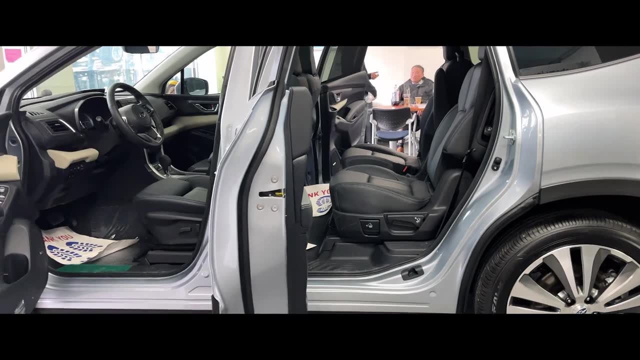 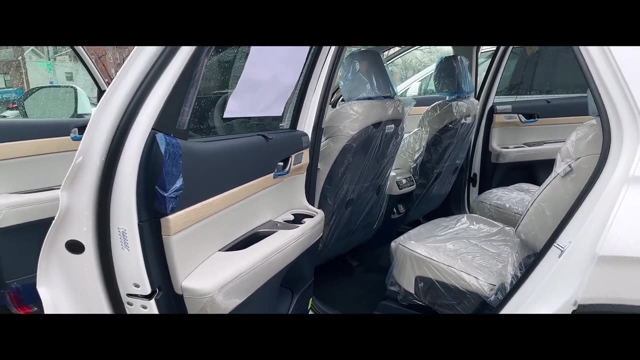 doors as being capable of opening wide almost to a 90 degree angle. but, based on our experience, no matter how wide your rear doors can open, especially if you are stuck in a very narrow positioning or especially like, let's say, theme park aquarium, where it's a packed day if you have cars parked. 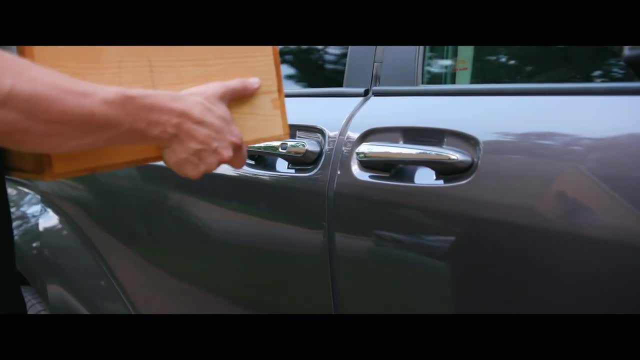 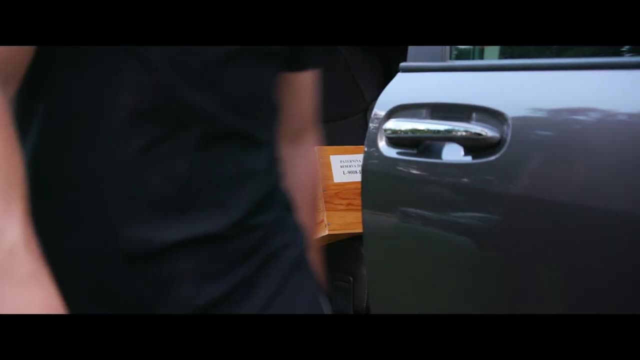 side to side. no matter how much, how, how wide your cars could swing, you're not gonna do anything with limited space, so that is why the minivan comes out strongly with sliding doors. the next topic: I want to talk about the third row space, because that's actually very important to us. 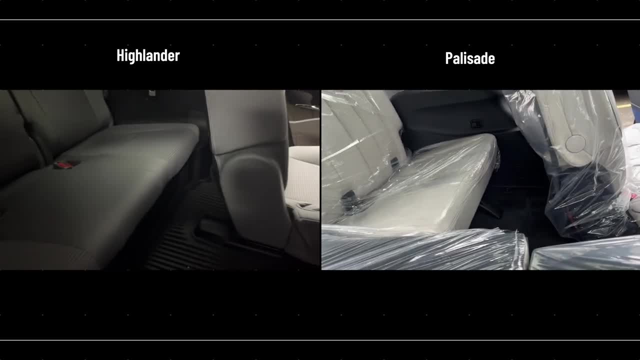 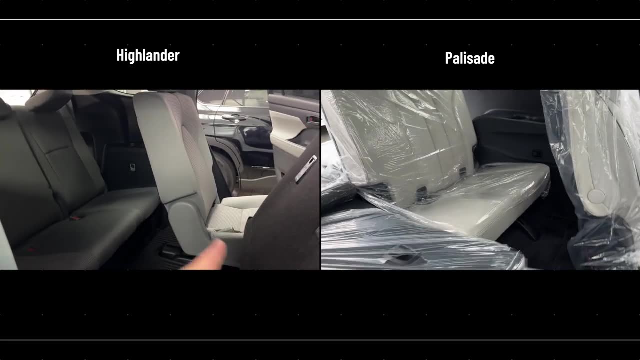 the reason I want to bring up the third row is the fact that all these cars that I'm mentioned before prior, they have like kind of like a raised floorboard on the third row so that even if you're sitting and you have enough leg room, your legs are when your feet are touching it's. 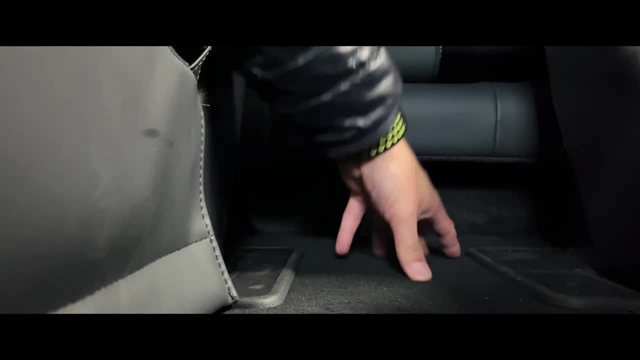 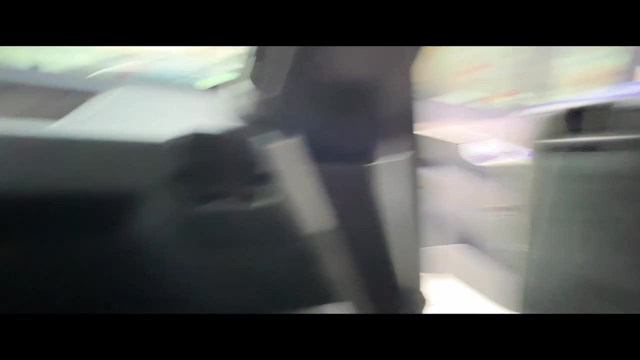 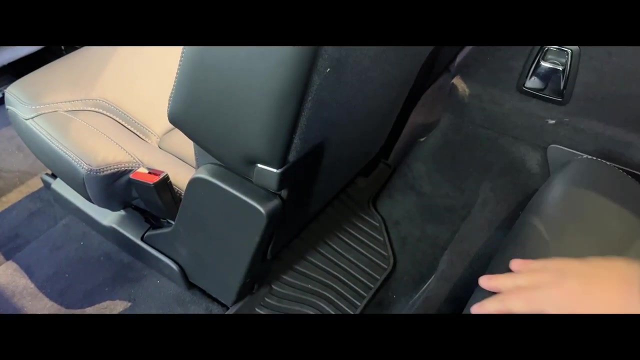 actually raised, so your knees are actually elevated as well. so that becomes really uncomfortable and i think those, the third row is actually really reserved for, uh, children, toddlers and, i guess, smaller adults, but my family, we're actually on the smaller side, as you can tell, so it could work. 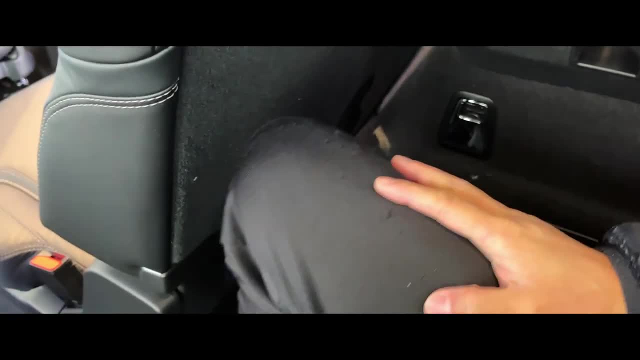 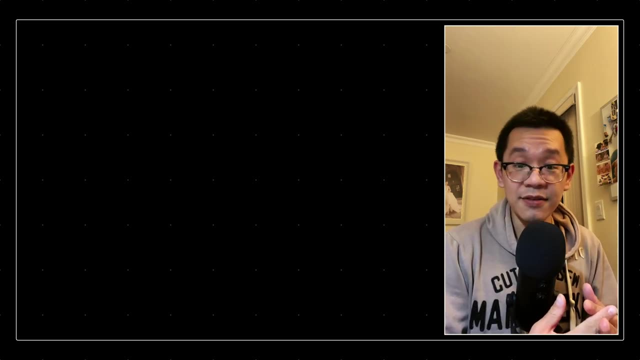 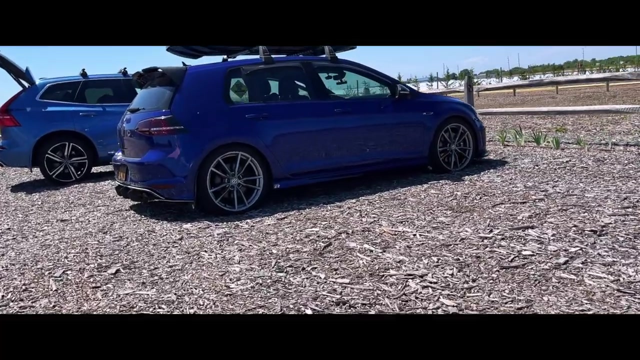 but really on a longer road trip i highly doubt it's going to be comfortable for any of us. we also learned from the past that having two cars is very it's it's a hassle, especially if one car is leading and the second car has trouble. for instance, to be specific, my dad was driving my vehicle, the 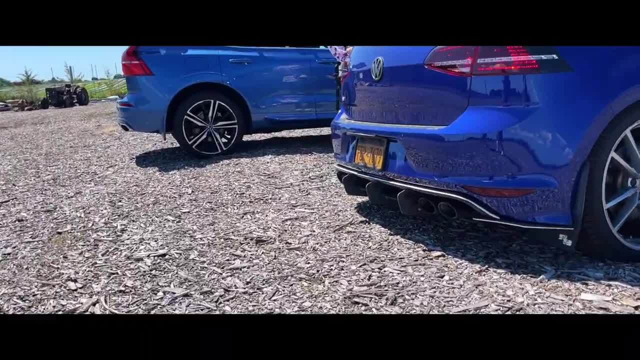 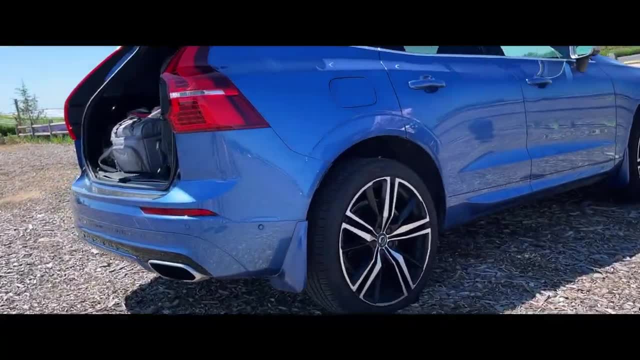 r back then and there was a tire pressure warning and he really wanted to go ahead and stop just to make sure everything's cool. the girls were sleeping, i was the lead car and from here for me to go ahead and get out to just check with him. um, it woke up. the 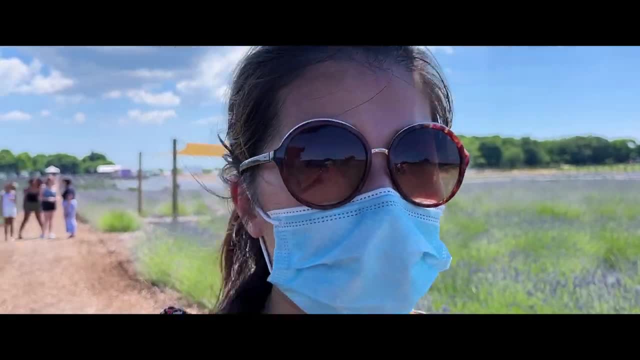 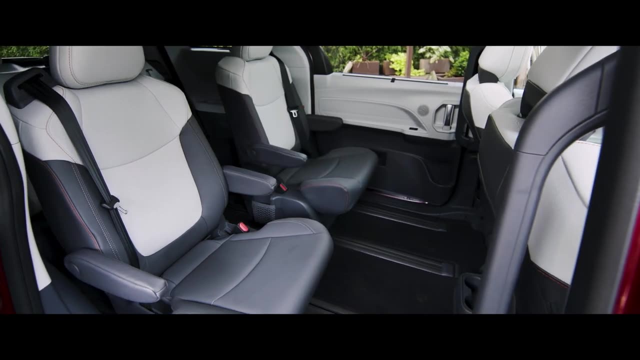 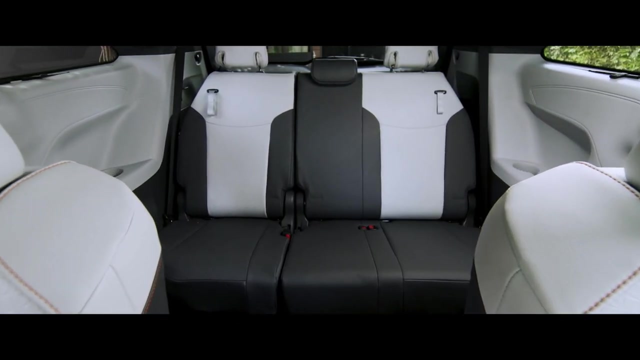 girl. so i think even before we got to our destination, we were kind of, uh, in a rough start, right. so having one car that's safe, reliable, having a third row, easily accessed and having good amount of um, third row leg room and also cargo space with the third row up is going to. 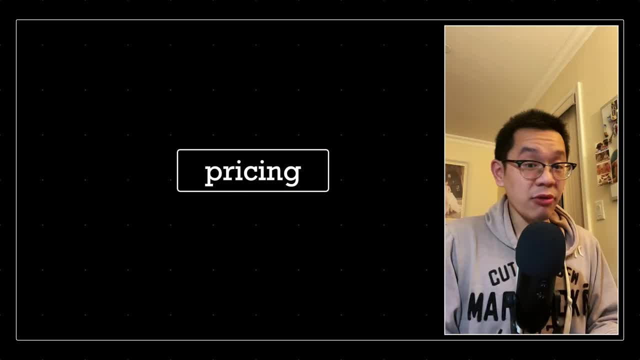 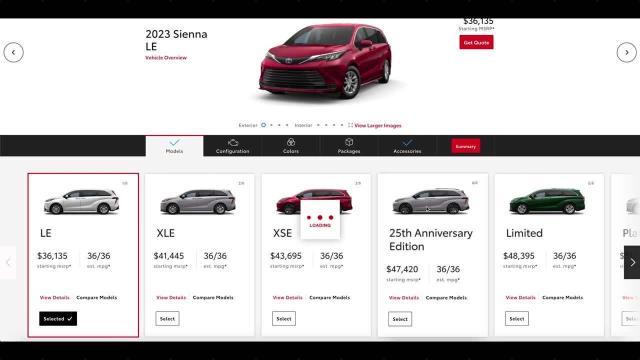 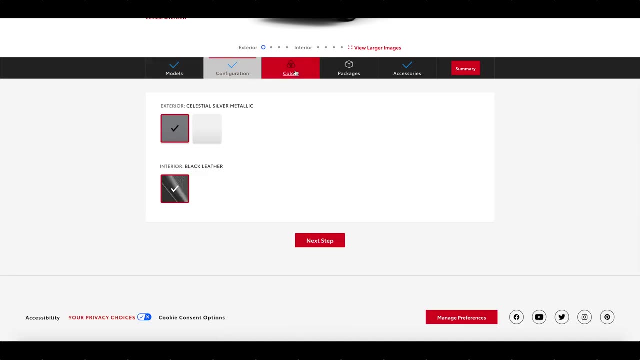 make life a lot easier now. lastly, i just want to talk about pricing and our budget. the sienna is actually above our budget. i really, really want to go ahead and keep it sub 40s, but due to the limited demands, due to, um, just overall market, we decided to go ahead and 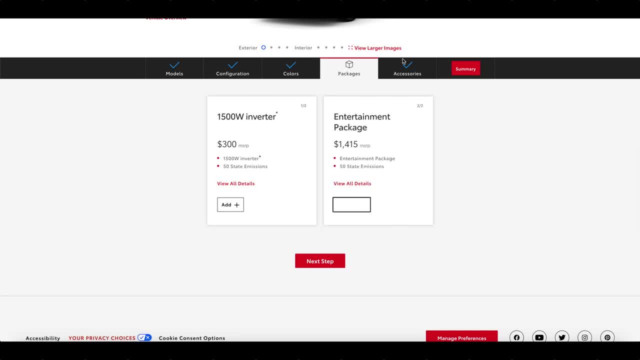 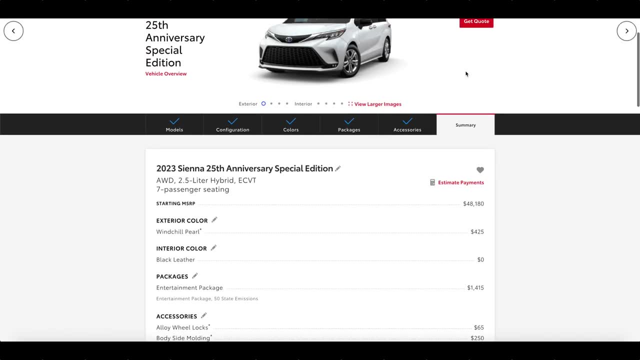 order a trim or two up from our budget, and that's why it's landing us in the 50 000 range, and from here all these other cars are either sub 50s or mid 50s. right and with tax, this is going to be a 60 000 vehicle. so thinking about that, it's like it. it puts me into another thinking perspective, like should, should we do it or should we not? and that's why we also considered the tesla model y, which, even though it has a seven seater option or third row option, i wouldn't consider a tesla model y with. 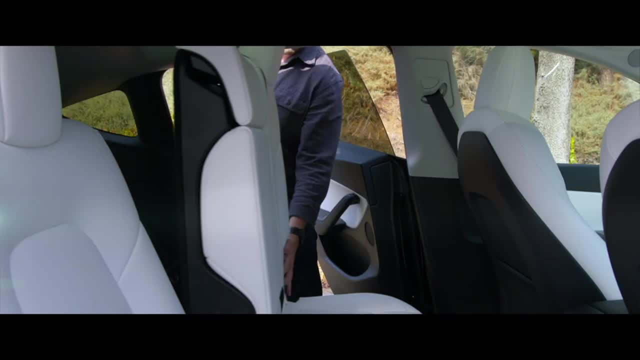 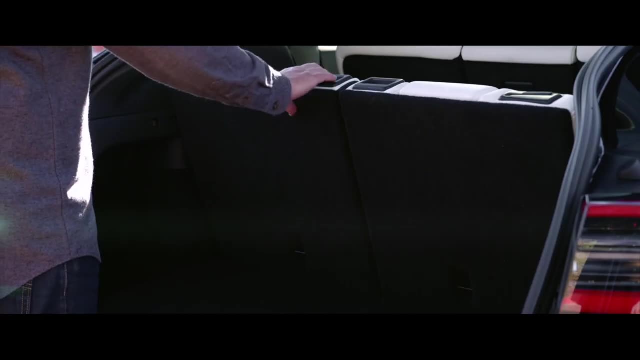 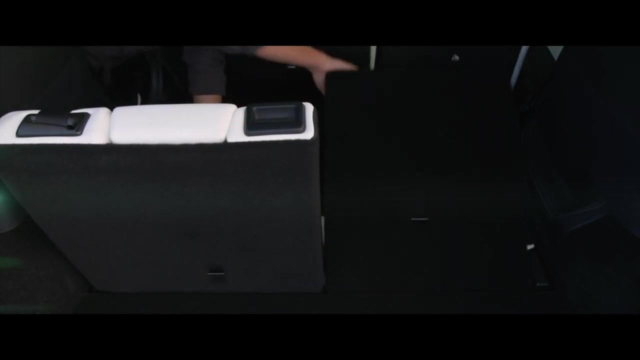 the third row, because i think that's completely, uh, irrelevant in terms of having a third row as any type of options. it's just so close to the rear cargo hatch and your, your head, basically reaches the sloping roof. that, um, i just don't think it's. it's worth it, but the tesla model. 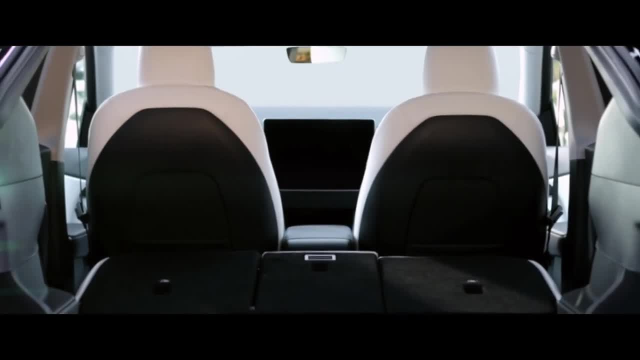 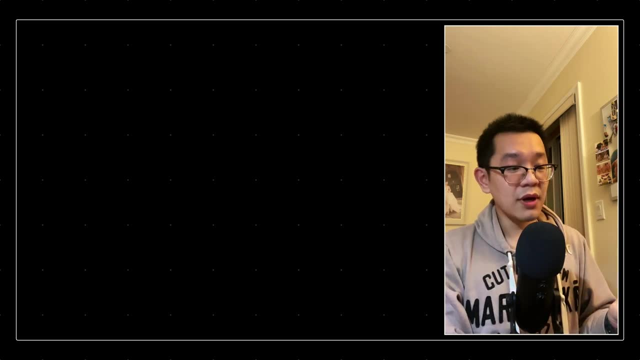 y is an option for us technically because it puts this car, even though it's sub 55s, it puts this car, after tax credits, to mid 40s. but along with that, if we're spending so much on these cars, why not consider it mdx and why not consider it xc90 and the gx used, certified, pre-owned? and that puts you. into sub 50s as well. so that's why we're also considering it and again, i wanted to go ahead and consider sq7, but completely, completely out of our budget. on the other hand, what other cars can you get in mid 50s? well, you could get a x3, the facelifted x3 with the b58 you could also get. 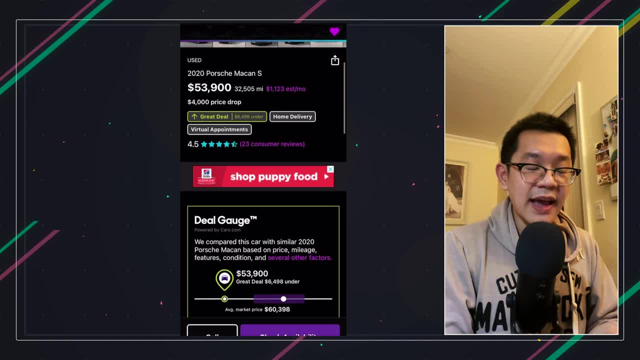 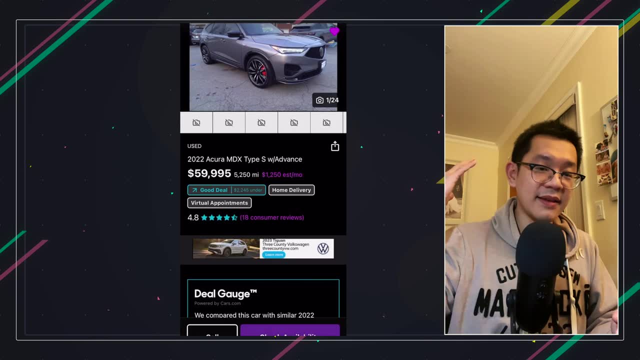 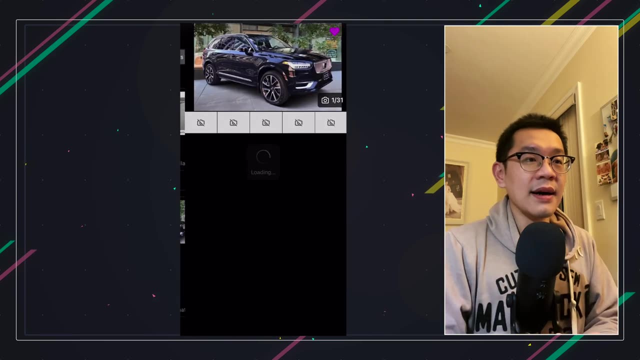 a used macan. uh, all this is kind of like my sport or my car enthusiast mind, talking to me kind of like devil's advocate, you know um. but moving on, i just want to kind of summarize everything, uh, and think which of these cars will benefit us in the long run and which of these cars hit every one of these criterias. well, it's either the sienna, the highlander and that's it, because those are the gas efficient ones. they're running the 2.5 inline fours. they're the bread and butter engine for toyota that they put on almost every one of their hybrid vehicles. 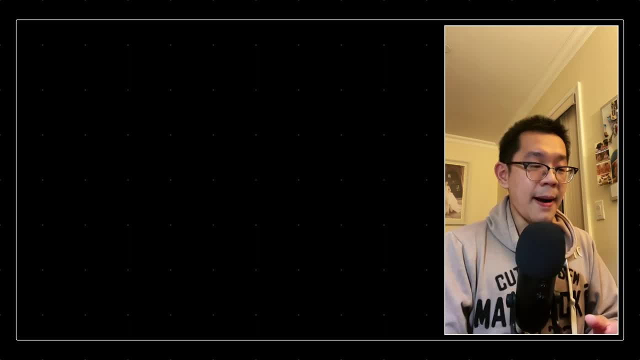 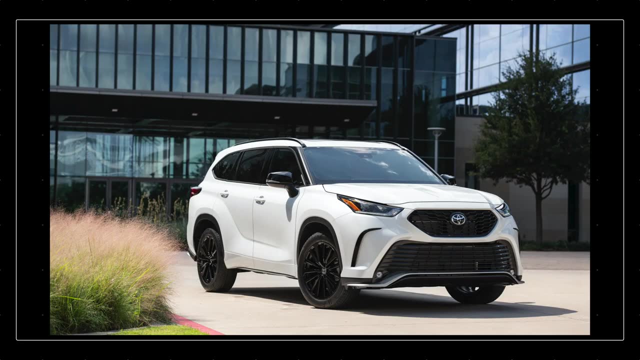 even in the lexus, too, in the new lexus line um. but there's something about the highlander. even though it looks nice, especially with the 2023 facelift, it look, it definitely looks more aggressive. however, with the rear seats, i just don't think it's possible. the 2023 highlanders. 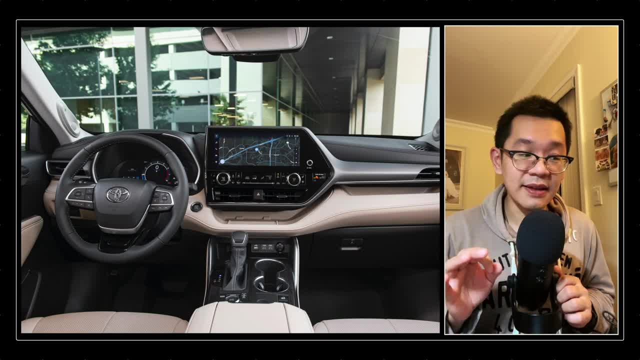 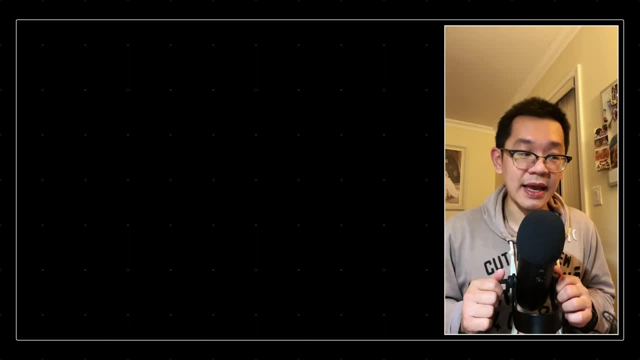 have a new infotainment system and i have a huge feeling that the sienna is following its footsteps next year, if not 2025. so i'm not sure if it's going to be a good year for the sienna or not. i'm pretty sure the sienna is going to get a revamp for the 2024, so as a 2023 model that we're 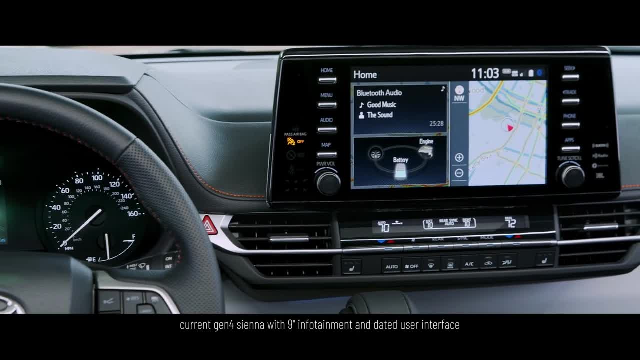 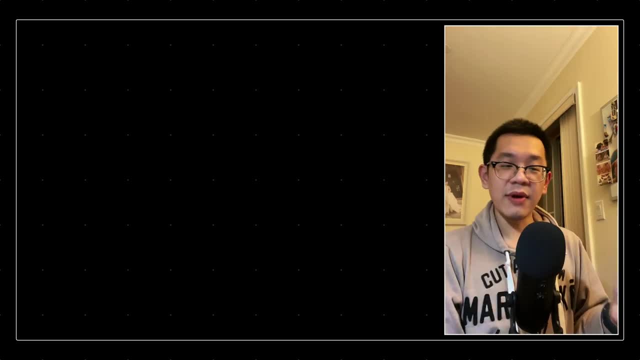 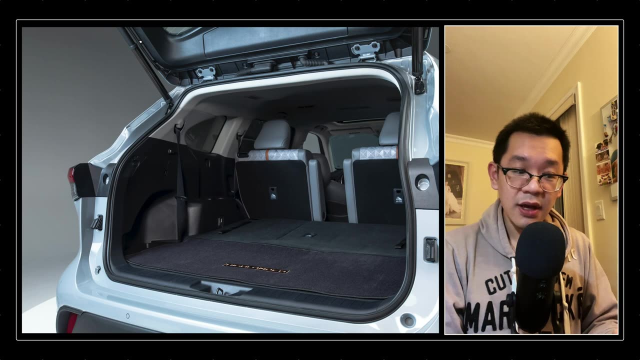 getting. that's not even in here. we're entering in an orderly dated infotainment system, so that's a kind of like a disappointing or a downer. now you can kind of argue: hey, the third seats are the third row seats are, um, gonna be there for, like kind of in a pinch situations where you really 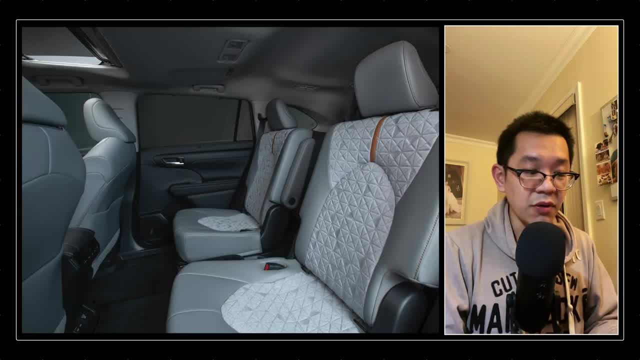 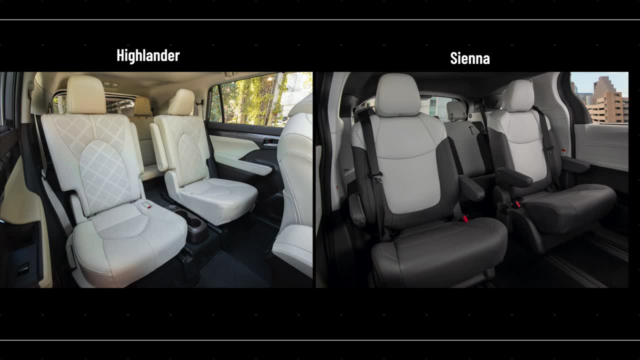 need them. for the most part, you're with your family with you, i'm with my two girls, and then from there the two rows work pretty well, but at the same time, though, i really want my family to be comfortable when they're riding with me. so the third row, especially with the third row cargo space, it's what's. 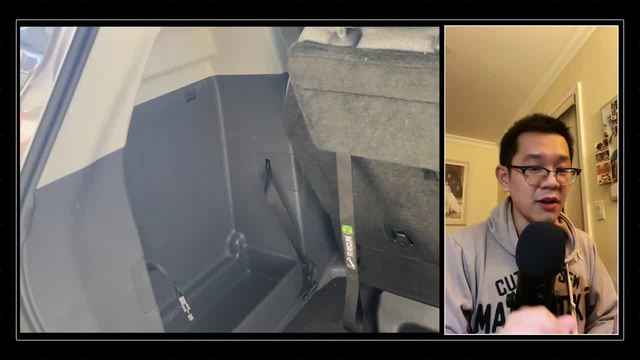 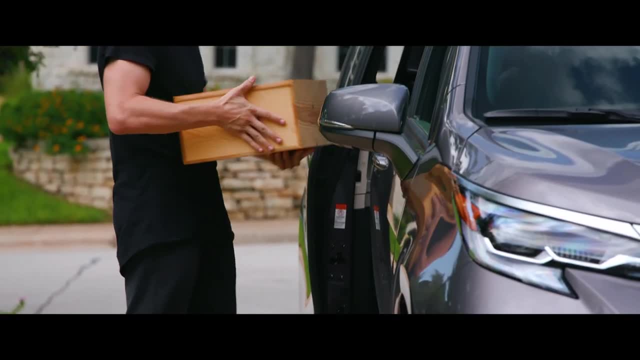 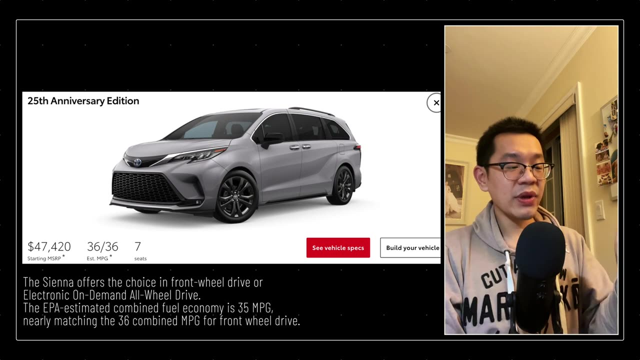 getting uh kind of driving it all home right: a minivan, minivan, minivan, especially with the sliding doors and with the hybrid we're going to talk about i. lastly, the epa gas mileage: 35 miles per 30, 35, 35 miles per gallon combined for the sienna, we'll overdrive. 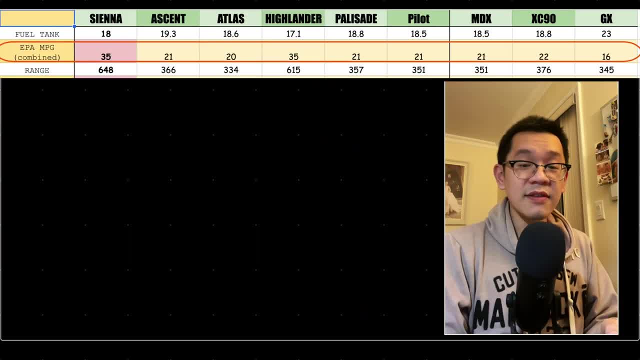 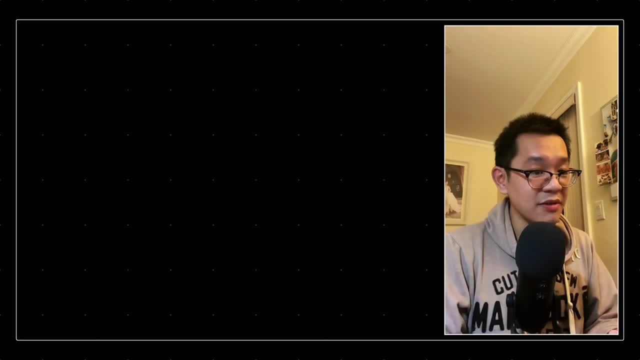 and also the highlander. all the rest of these vehicles are running sub 20s, right of course. granted, they have more power. they sound much nicer, especially with the atlas, especially with the gx, with the v8, the vr6, especially if you throw in a resonator. delete. 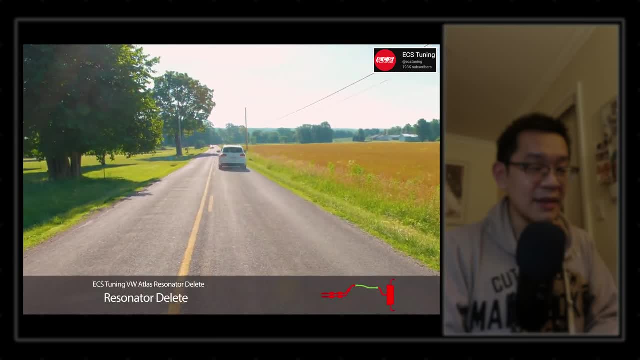 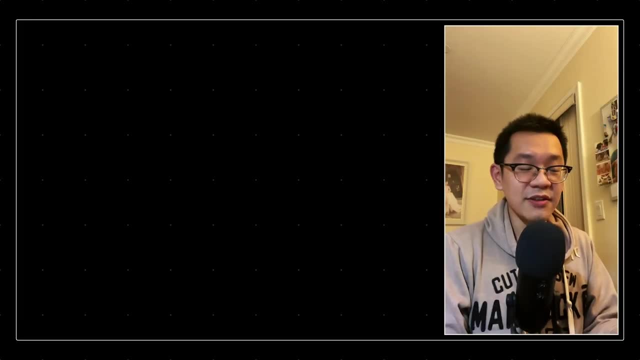 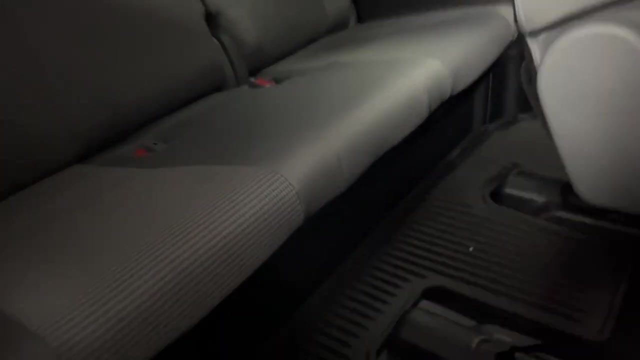 it's going to just open up the sound it's going to be, it's going to sound amazing. having said all that, i think it knocks every, each one of these vehicles out, besides the sienna and the highlander. but the highlander without the third row, uh, the lack of leg room, a lack of cargo. 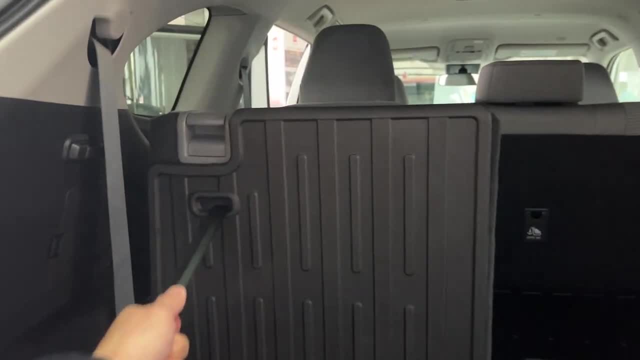 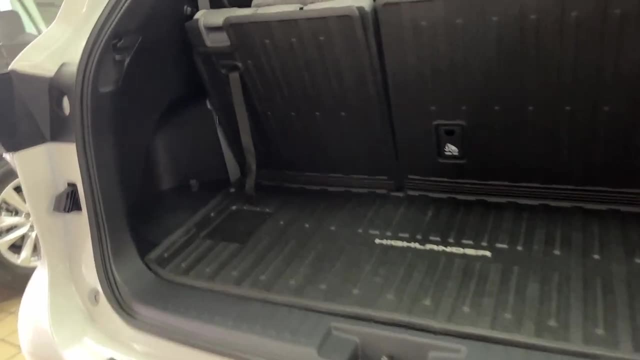 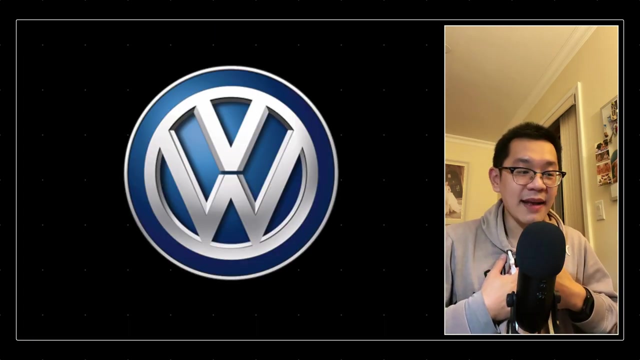 space at 16 cubic feet with the third row up. it's not. it's not going to cut it, especially with the stroller, especially with luggages and everything on a road trip. it's not going to work. so from here, the sienna is a top choice. but being a volkswagen owner for the past 10 years, 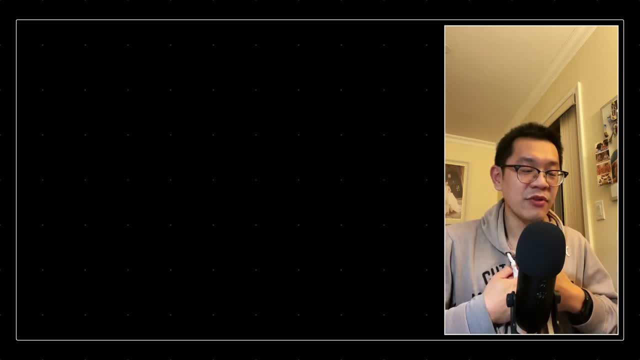 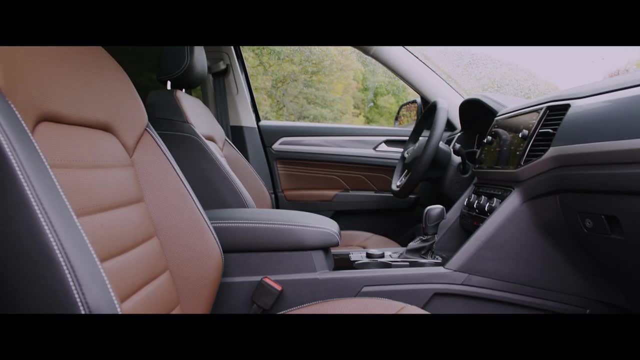 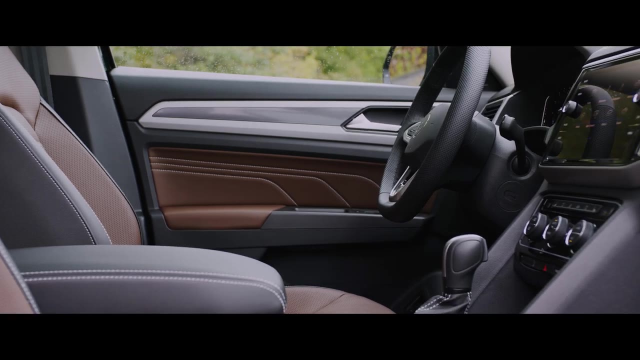 plus, um, i'm just very proud that the atlas was one, the one car that made me rethink, that made me go ahead and speak to my wife and say, hey, maybe the sienna isn't, we don't need the minivan at all, maybe maybe we could do make do with the atlas. right, the atlas will. it's huge, it has a really 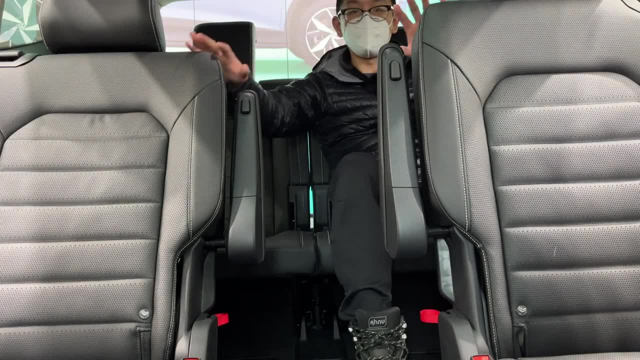 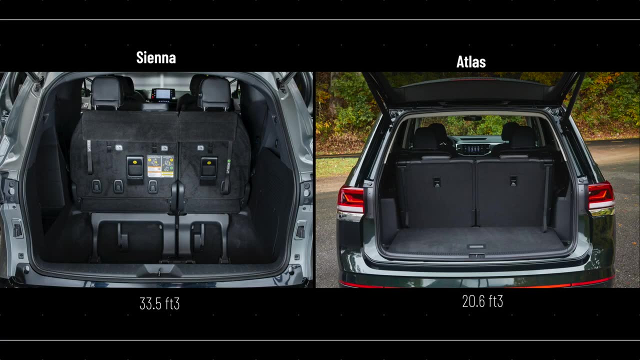 good and impressive third row and just a little bit shy of the sienna specs. it has good cargo specs. it has a good cargo specs. it has a good cargo specs. it has a good cargo specs with, especially with the third row up: 33.5 in the sienna versus 20.6 cubic feet. 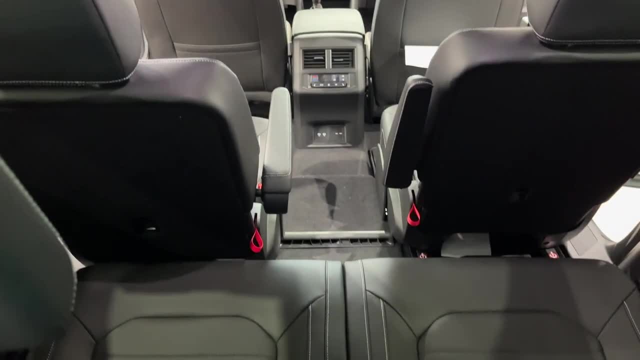 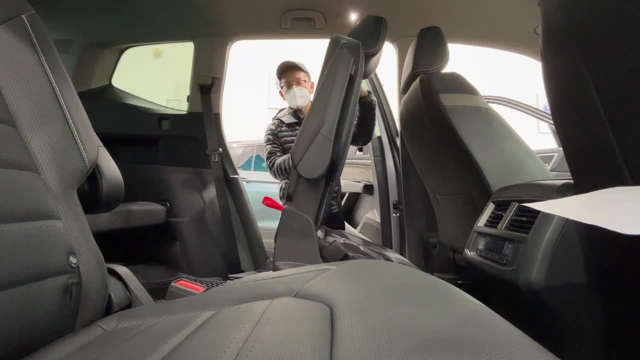 it has nice captain's chairs and most importantly, i think with the captain's chairs the atlas is the only car or the only stv that could kind of lift up the whole seat with a car seat attached to it and have the third row passengers go in and out, so you don't have to. 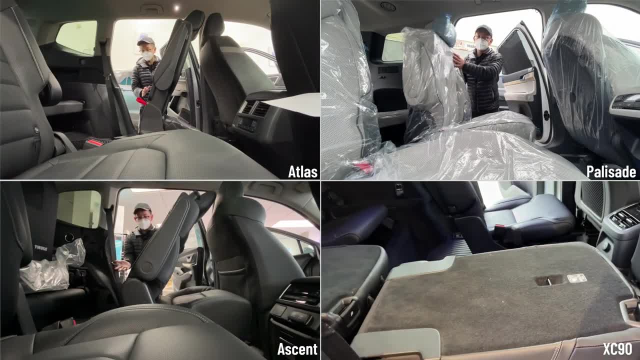 go ahead and fold down if you have a car seat, it basically um inhibits your captain's chairs from folding down, so you don't have to go ahead and fold down if you have a car seat. it basically um inhibits your captain's chairs from folding 90 degrees or even folding at an angle because of. 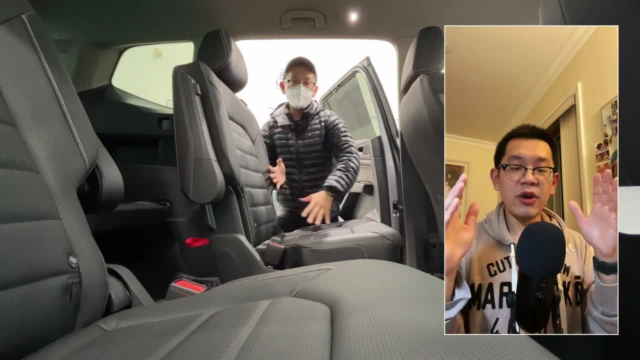 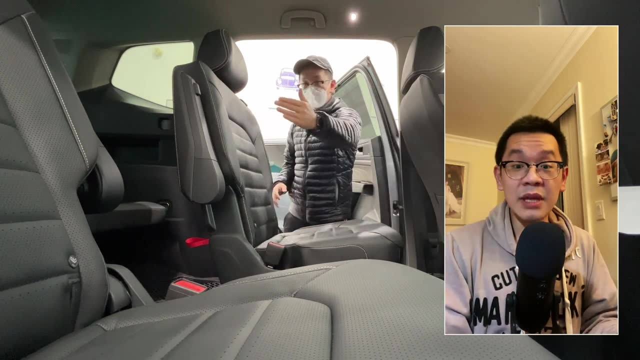 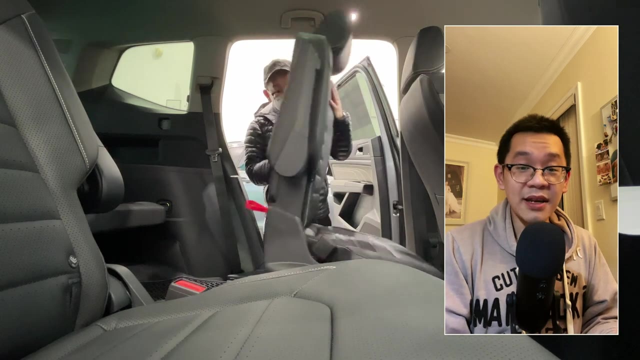 the car seat, but the atlas, the engineering of it, you're able to kind of tilt the whole seat upwards towards the drivers or passenger and from here just make everything work. so atlas from here really was impressive. it made an outlasting impression on me leaving the the dealership. 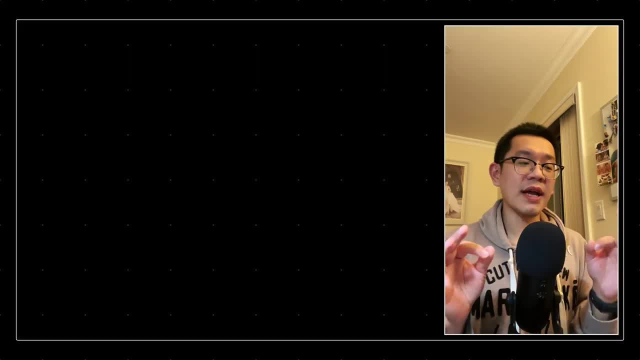 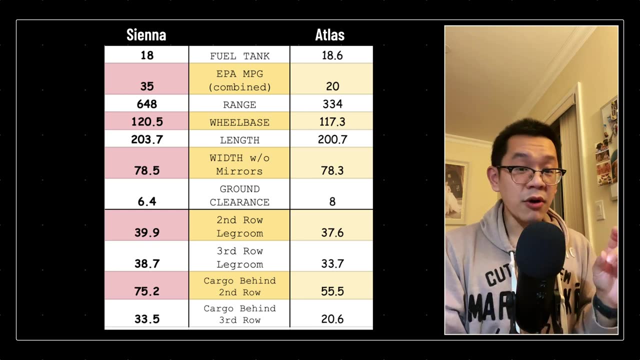 and it had me rethinking. but what really made me go ahead and decide on the sienna is the fact that it is only four inches long and it's not a lot of space. and it's not a lot of space and it's not three inches or three inches longer than the atlas, because the atlas is at over 200 inches in length. 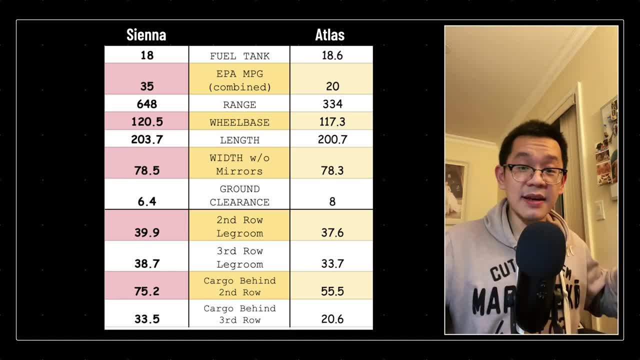 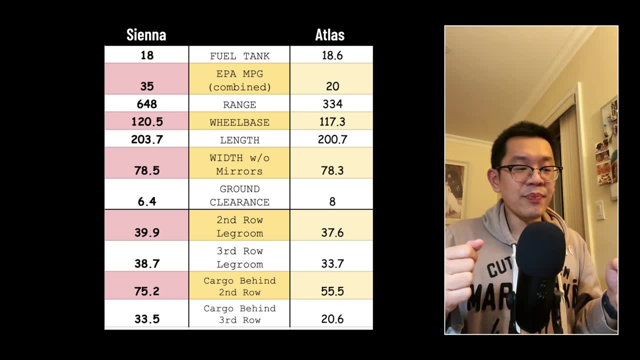 in terms of width they're pretty much the same. i believe the sienna has maybe a little bit bigger mirrors, so it's a little bit wider, so getting into our driveway might be a little bit harder. but i think, with the atlas in terms of size, i might as well go for the sienna. 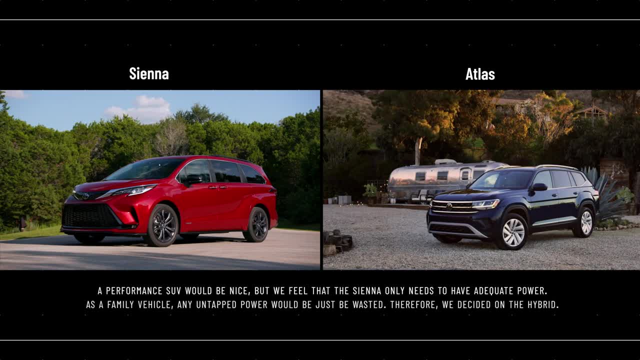 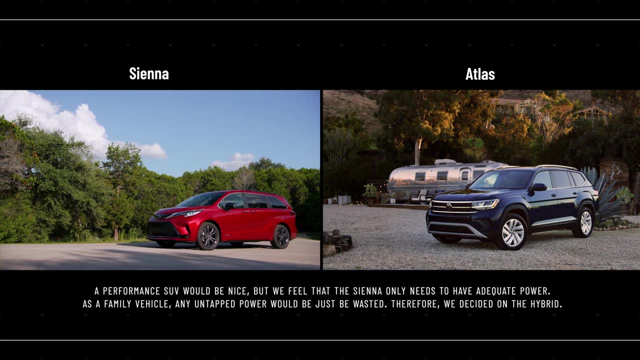 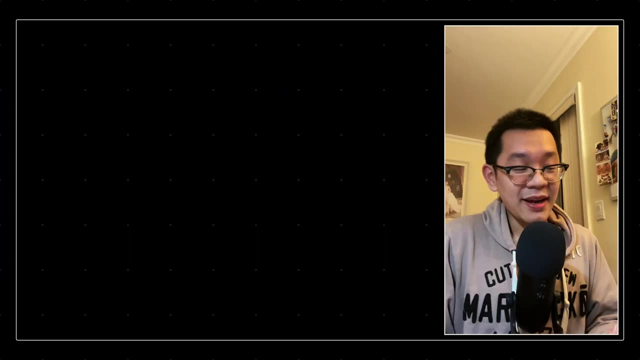 if you're going for a vehicle that big and you're averaging 20 miles per gallon combined, i might as well really go for the sienna, because you're getting at least 15 miles more per gallon than the, than the vr6 equipped vehicle. i have a feeling, if i'm driving really